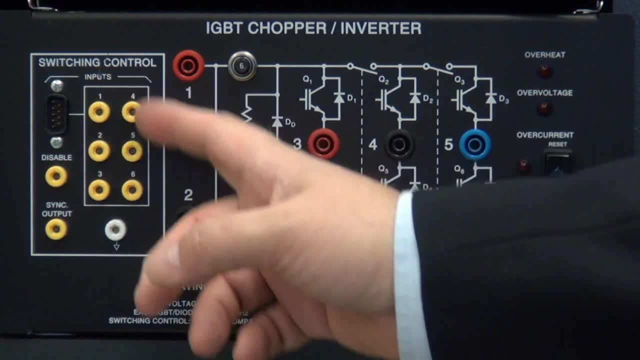 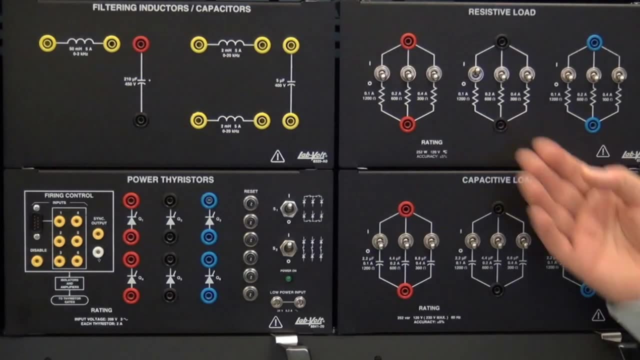 There is protection against overheat, over voltage and over temps on output. In addition to that, over current, all of the gate signals can be observed on an external scope or using our data acquisition system. a variable resistive load allows seeing the influence of the load on the. 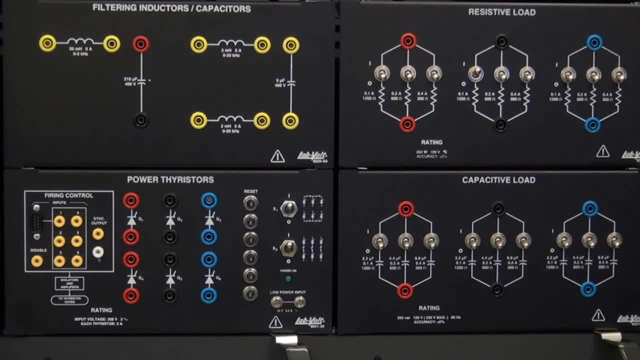 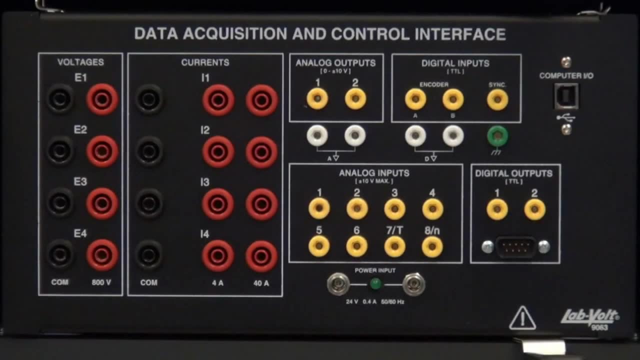 circuit and a variety of filtering inductors and capacitors, allows switching frequency to be varied from 400 hertz up to 20 kilohertz. the data acquisition and control interface features four high voltage and high current inputs that are fully optically isolated as well. 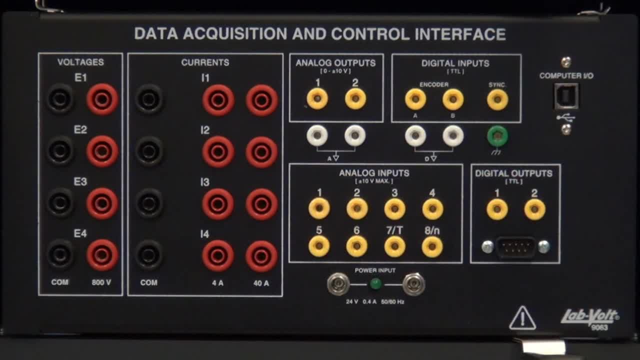 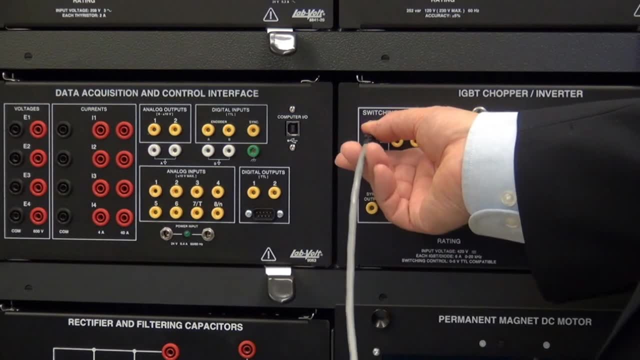 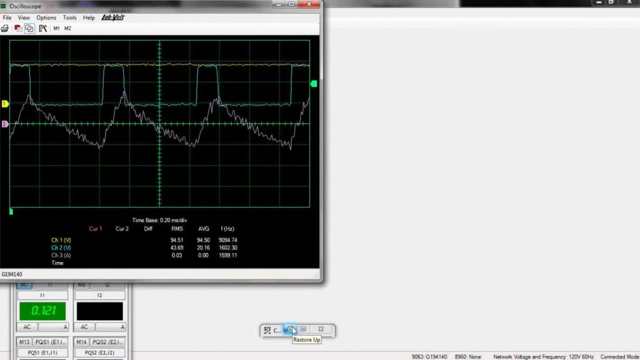 as enough analog inputs to be able to observe all of the gates and triggering signals. the control of the igbt gates is as simple as connecting the inputs of the gates to the output of the data acquisition. the system also allows you to take control of your transistors. 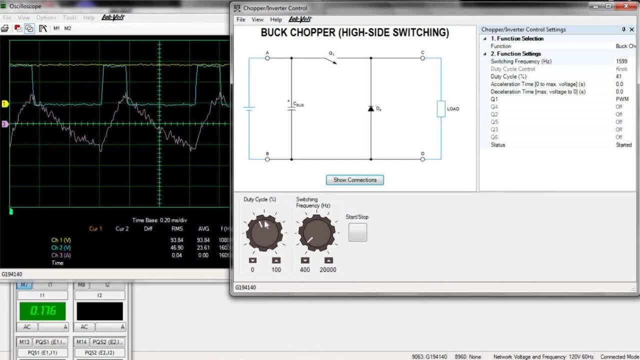 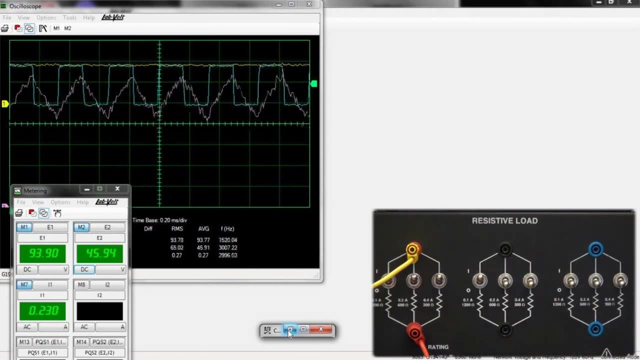 by controlling things such as the duty cycle, the switching frequency, acceleration and deceleration time, as well as selecting the configuration from a multitude of different functions. Once connected, the data acquisition allows you to see all of the pertinent signals on the oscilloscope Using the four quadrant. 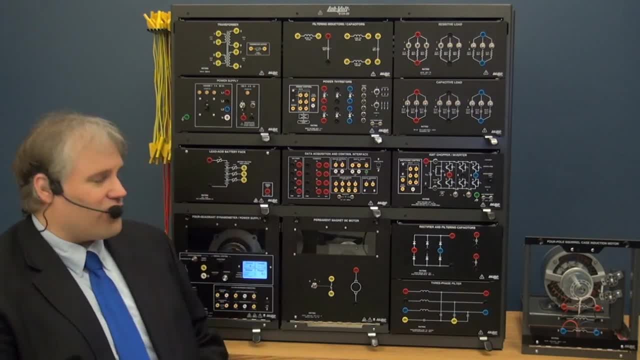 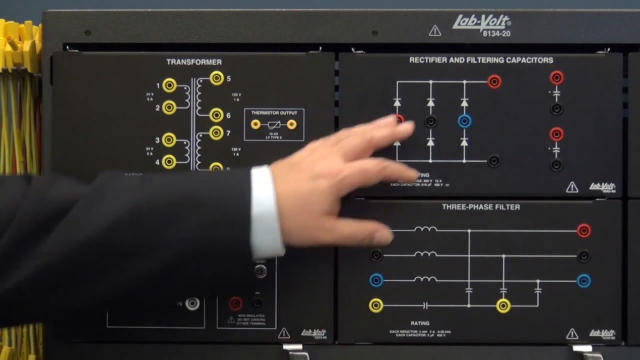 dynamometer to control the torque and the speed of the DC permanent magnet motor. the students will then create a buck chopper drive, a buck boost chopper drive and a four quadrant chopper drive. They will also do a DC motor control using speed and current feedback, Using the rectifier and filtering capacitors. 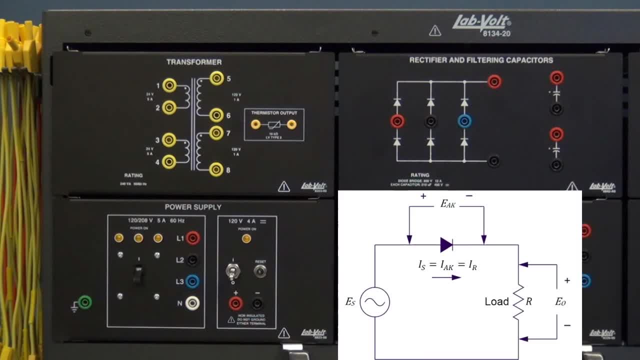 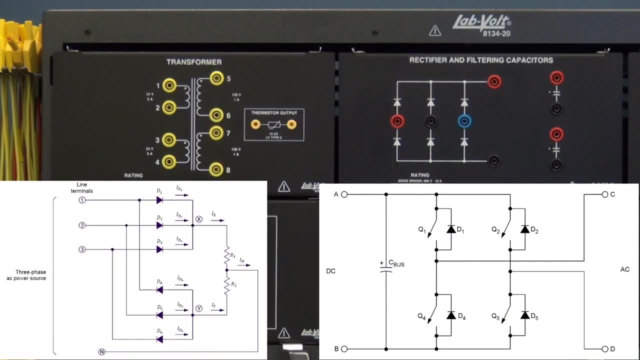 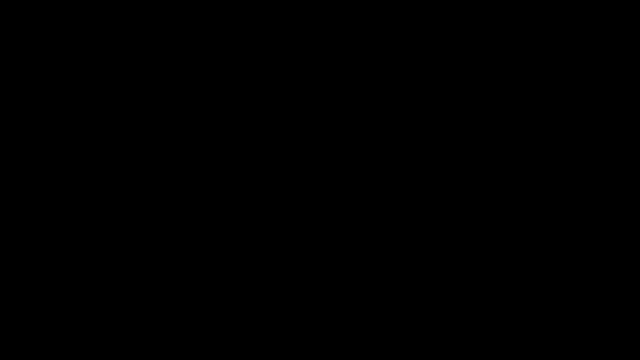 along with transformers. the students will then study power diode single-phase rectifiers, single-phase PWM inverters, as well as three-phase rectifiers, single- phase PWM inverters with dual polarity, DC bus and three-phase PWM inverters. The 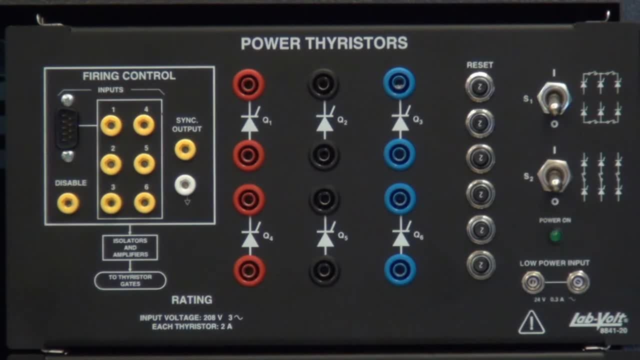 power thyristor module will be controlled with LVDEC as well. The individual SCRs will be controlled with LVDEC as well. The power thyristor module will be controlled with LVDEC as well. The individual SCRs can be linked together using two separate switches and the firing. 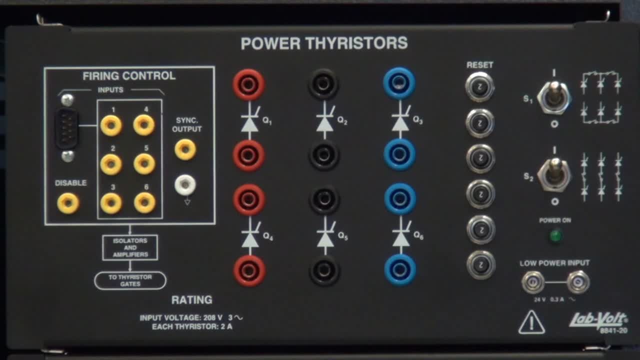 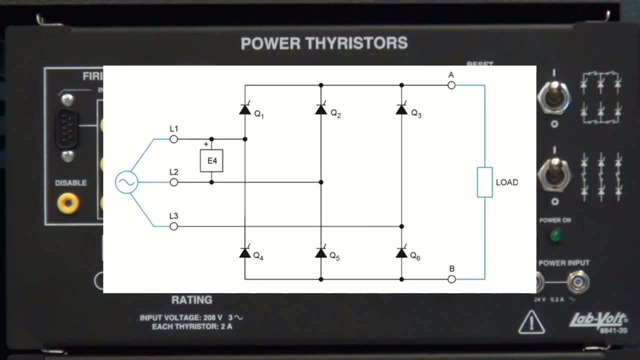 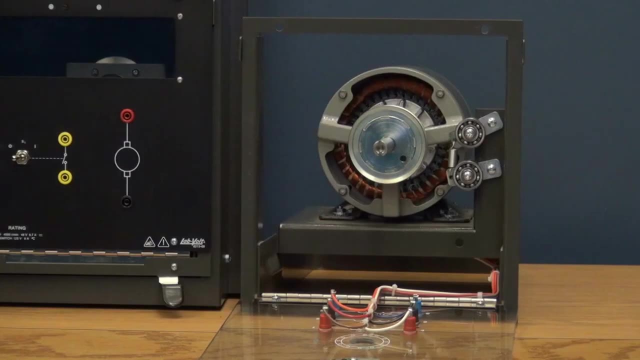 control. signals can be seen on the oscilloscope as well. The students will do study the power thyristor: single-phase AC power control, as well as three-phase AC power control thyristor, three-phase rectifier, inverters and solid-state relays Using the three-phase squirrel cage motor. the students will